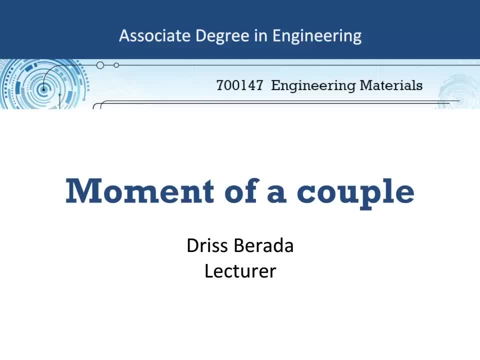 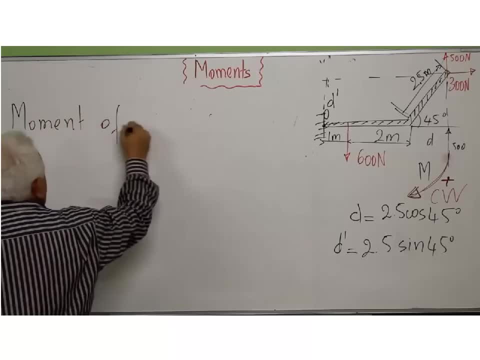 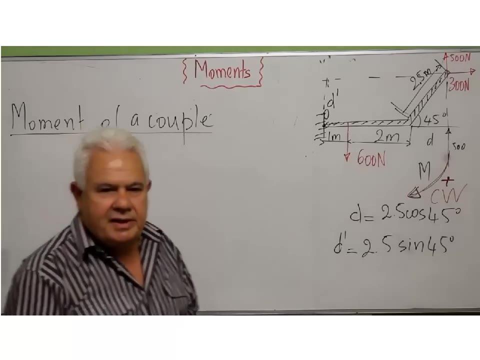 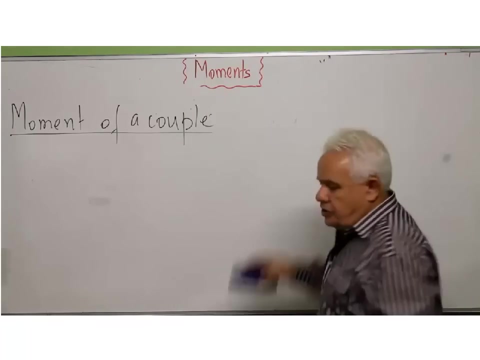 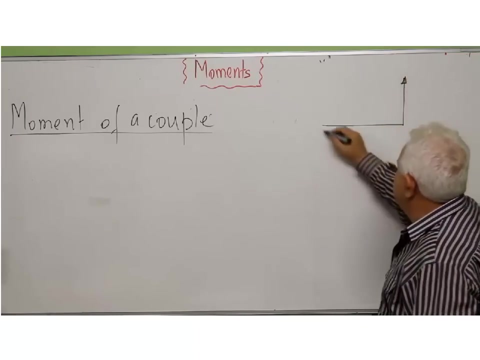 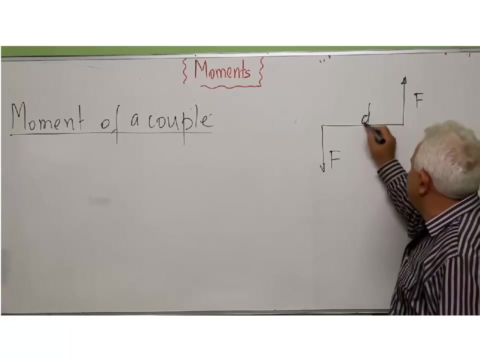 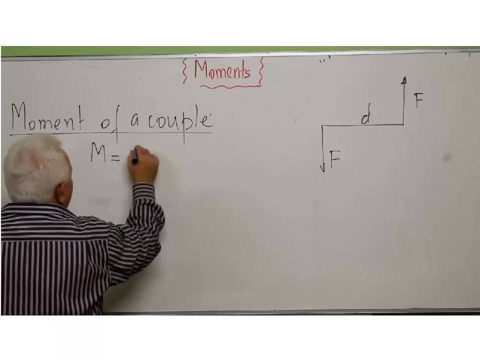 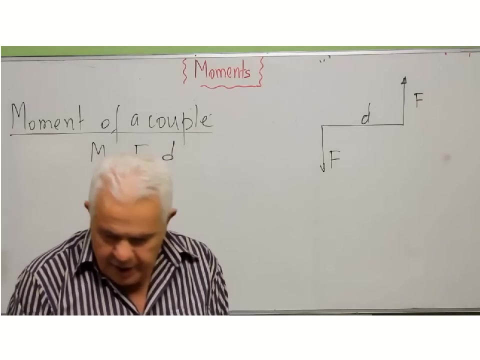 Welcome back to this series of videos. A couple is a system of two forces acting in opposite direction. Simple stuff. We have two forces but equals in magnitude. We have FF separated by a distance, D. In this case we define the moment of a couple. M is F times D, as we have seen before. I'll give an example. 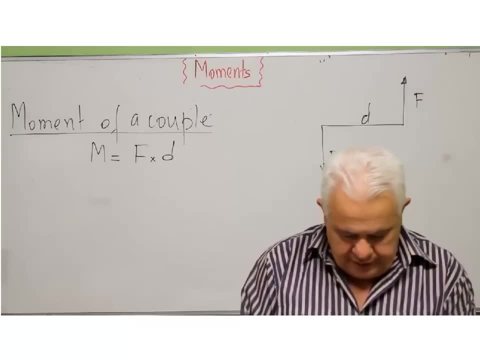 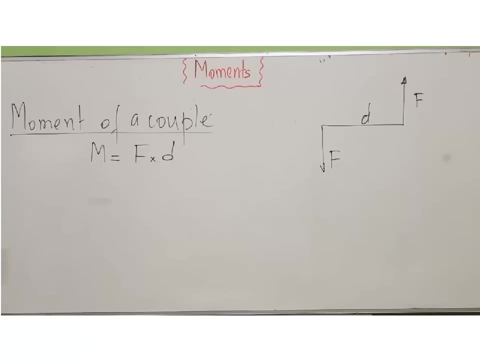 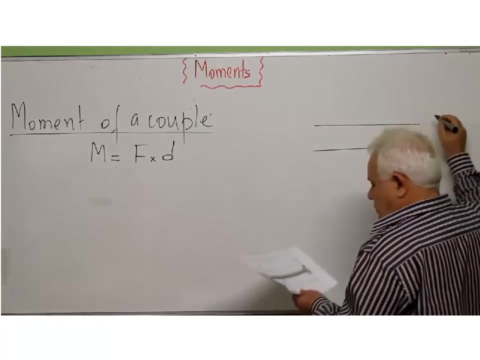 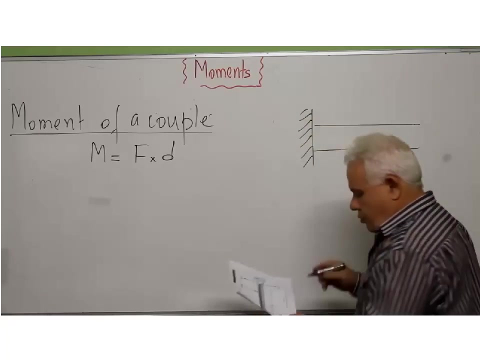 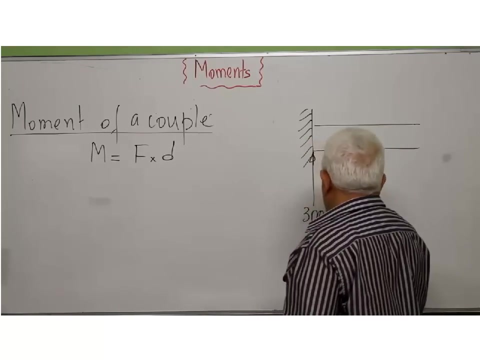 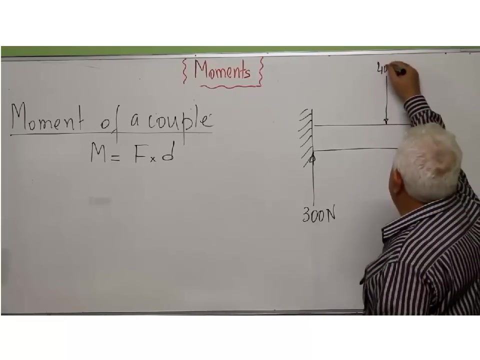 and I will conclude with this video. Suppose we have to calculate not one couple of moments, but we have this case in which three couples are acting on a bar like this. We have a bar here in which we have one force here of 300 newtons. Another one here is acting at 400 newtons. This one is acting. 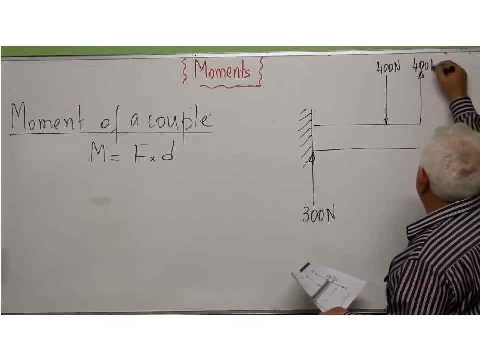 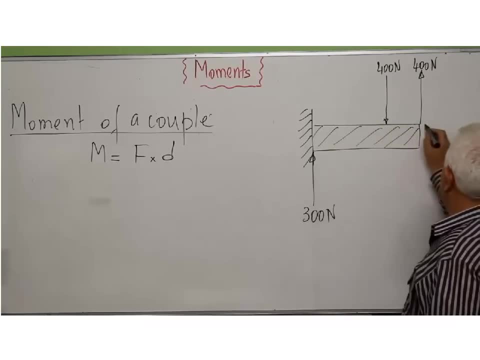 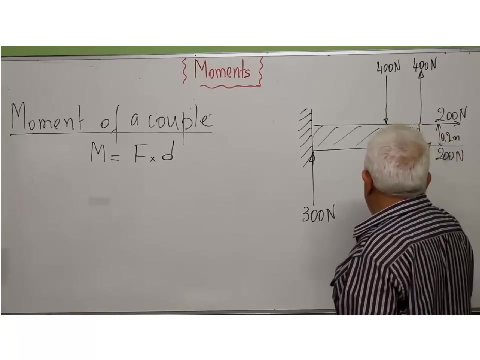 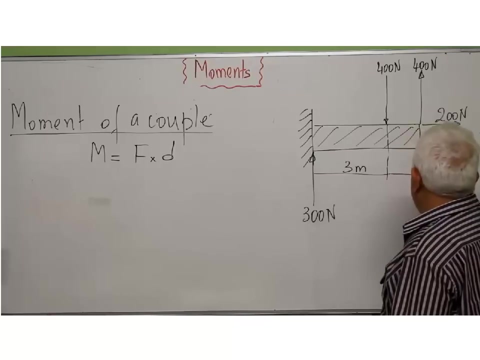 in the opposite direction. Another couple of moments here is acting in the opposite direction. We have 200 newtons. 200 newtons separated by a distance 0.2 meter. Here we are at a distance 3 meters, for example, And from here to here we have 2 meters. 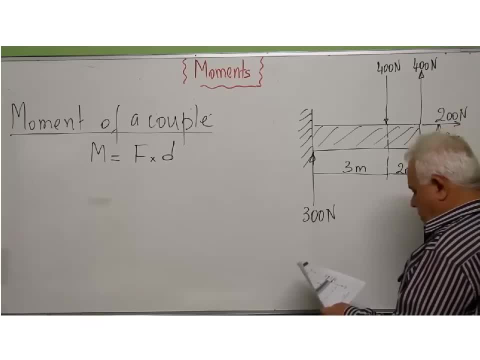 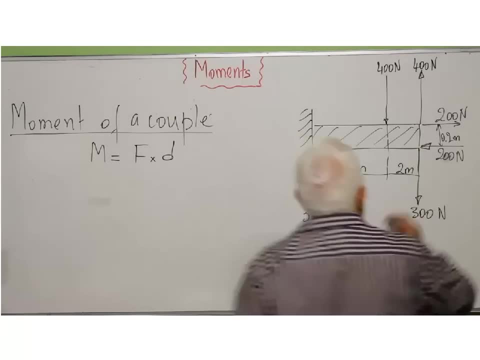 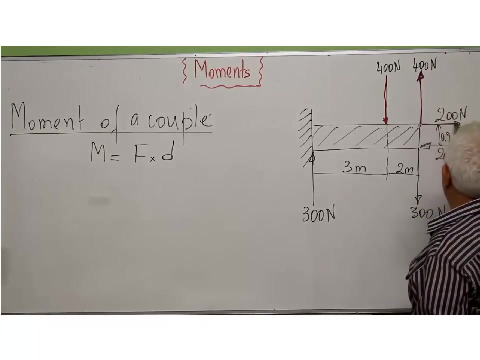 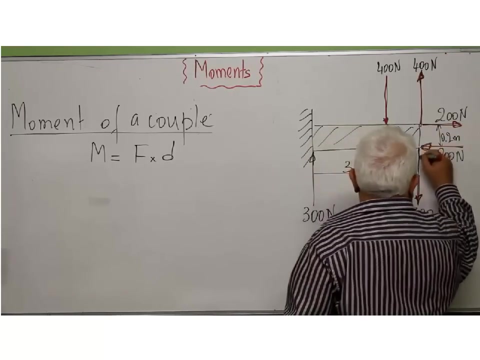 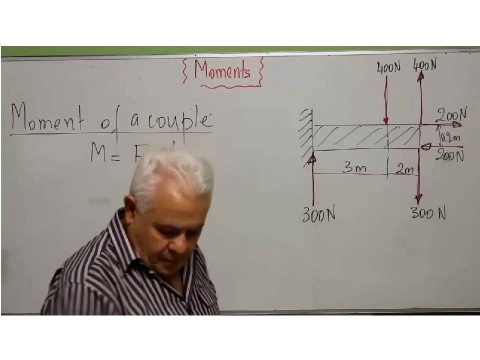 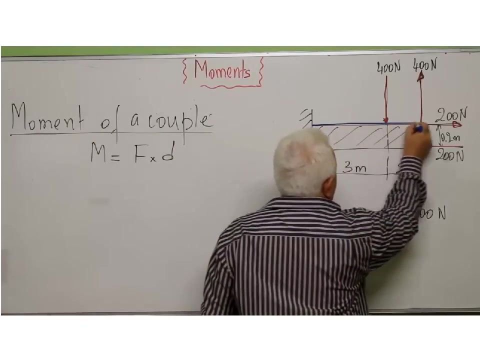 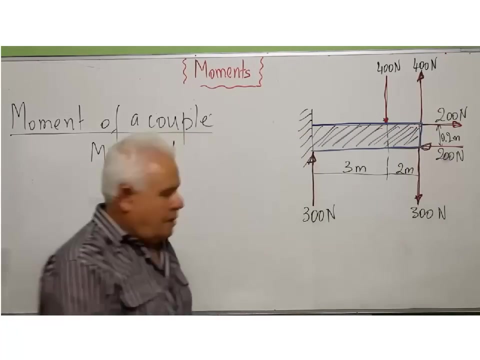 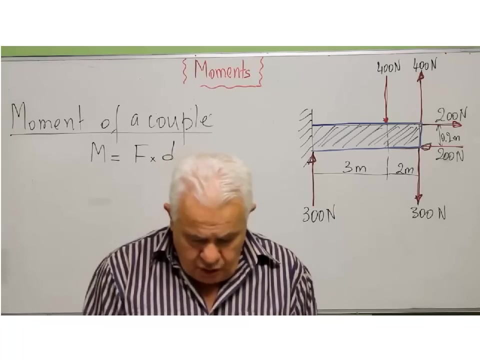 And the force of 300 newtons is applied. I'll just put them in red. So we have one force here, another force here, another force. Now we are out, And my system is this bar. So, like forces, the couples, if we want to calculate the resultant couple of couples, 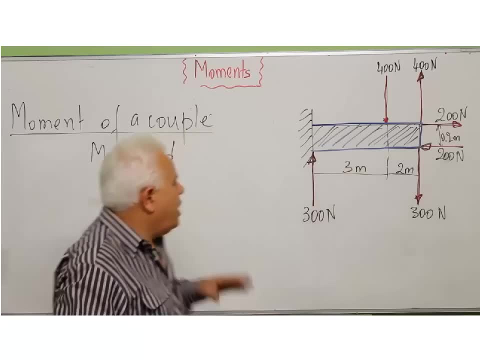 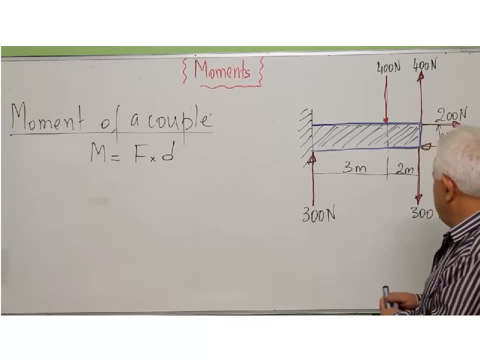 the resultant couple of all these forces. we have just to add them. But we have to choose before doing that. a sense of orientation, For example. if I choose this one, clockwise, it's arbitrary. You can choose any direction that you want. 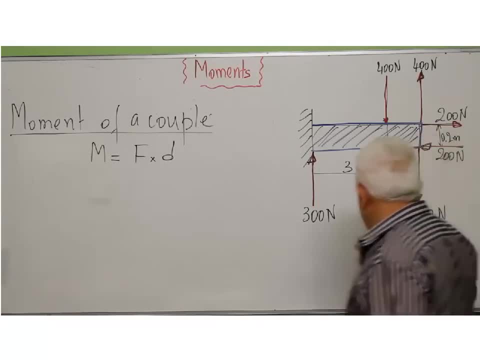 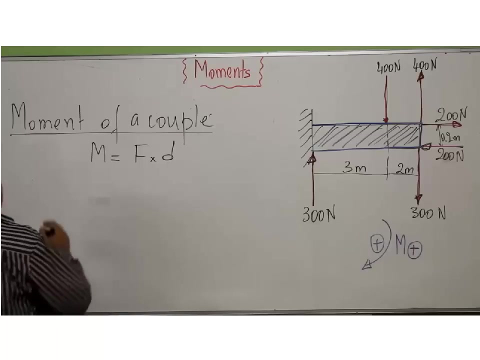 But you have to choose one. This, So all the moment the couple is turning Turning clockwise has to be taken as positive. So let's start. We have moments, The moment resultant of the resultant of these 3 couples. I've got this first couple of 3 handles. 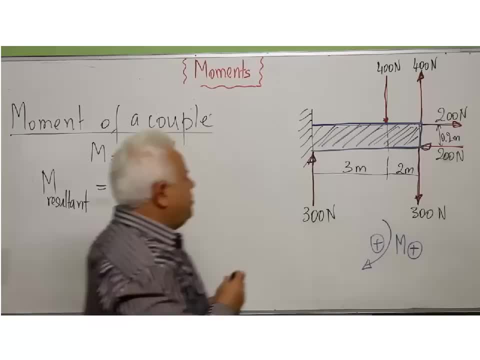 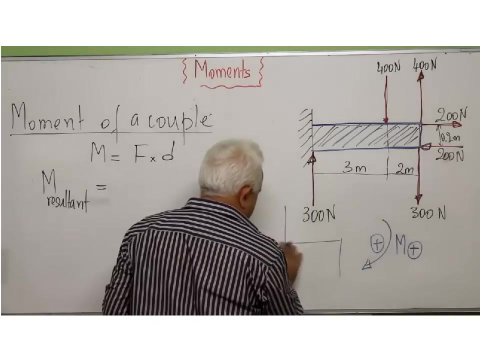 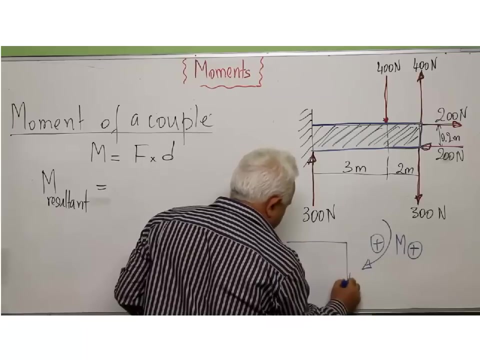 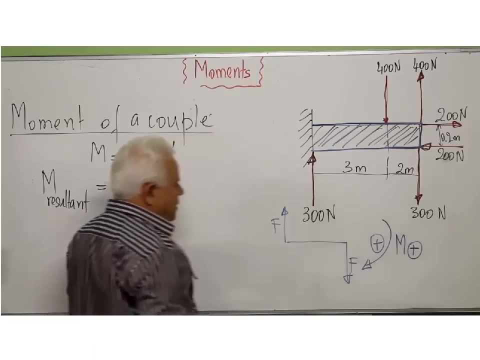 Second couple, 4 handles And the third couple is 2 handles. So this, The positive moment, just will be something active. for example, I have 2 forces like this: F equals in magnitude. This is clockwise In this configuration.